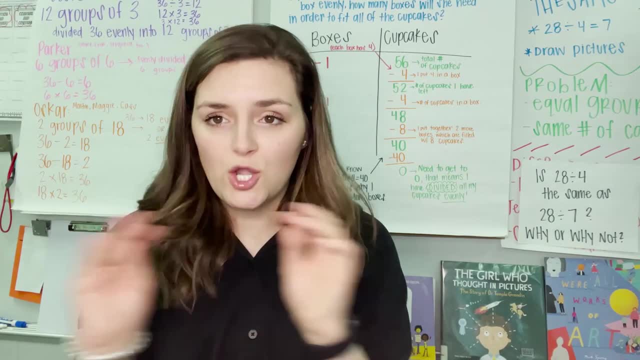 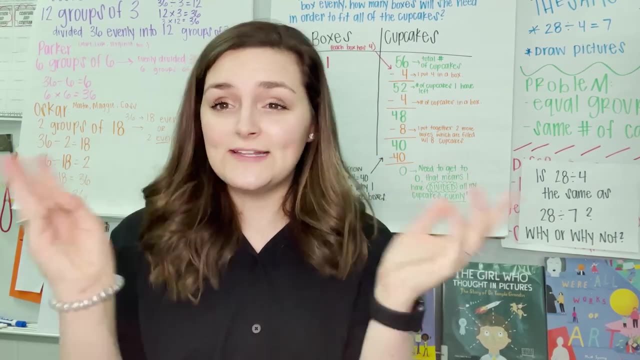 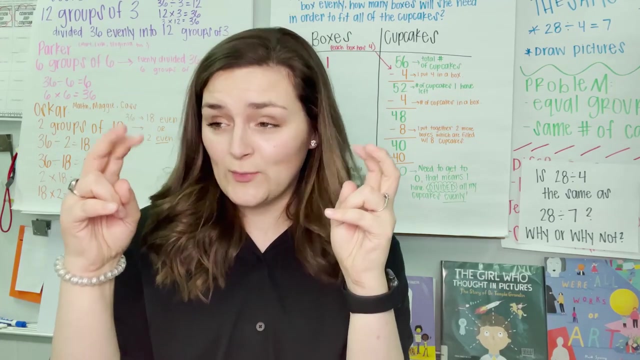 these classes that I lacked number sense and fluency, And at the time I had no idea that's what it was, And so numbers weren't connecting. And yes, like many of you, I plugged two plus three into my calculator. So I had consciously labeled myself as not a math person. And I, and it wasn't for me, And I remember. 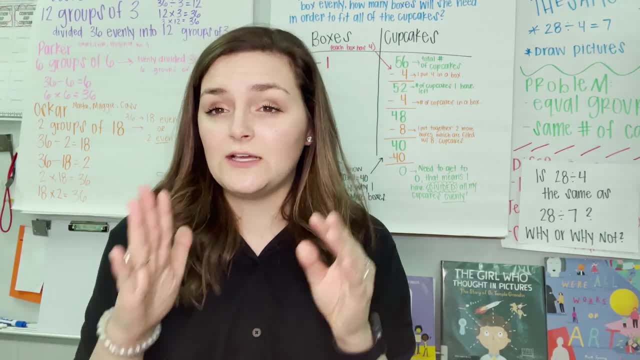 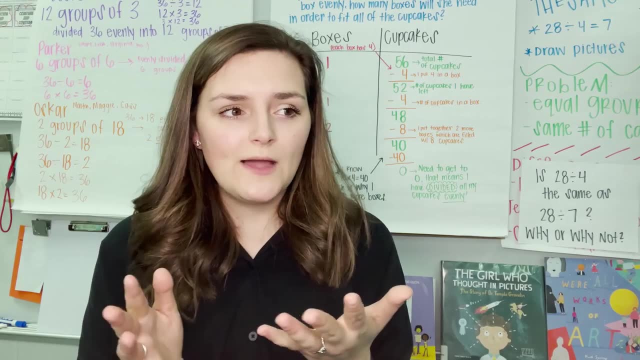 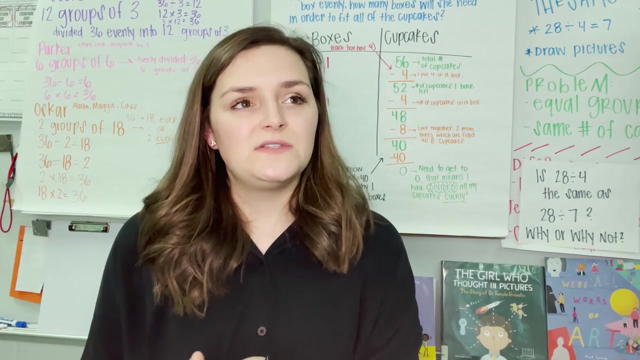 feeling like such a loser. when I was recommended to take a lower level math class for my junior year, after only taking honors classes since I was in middle school, I was wrecked. I felt like such a loser. But my junior year I got really lucky And I had a really awesome teacher And he took 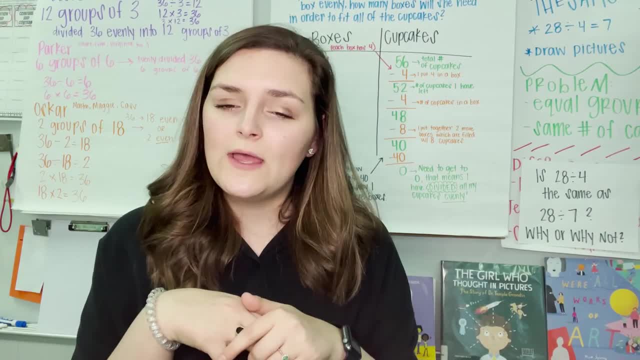 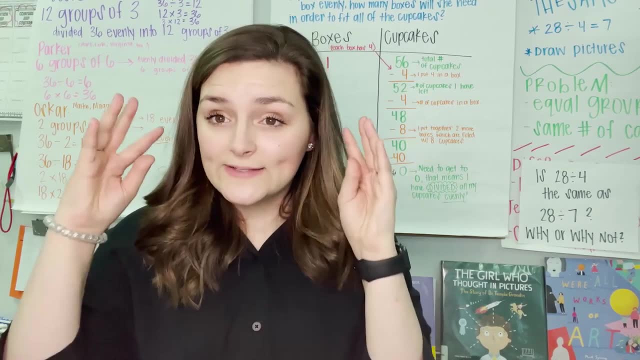 the time to make sure that we understood the concepts of algebra too, And he really made me feel like I could do math, even if it was for a short while, And so my confidence was boosted And my headspace was a lot different. And so flash forward to college and I was knocked down. 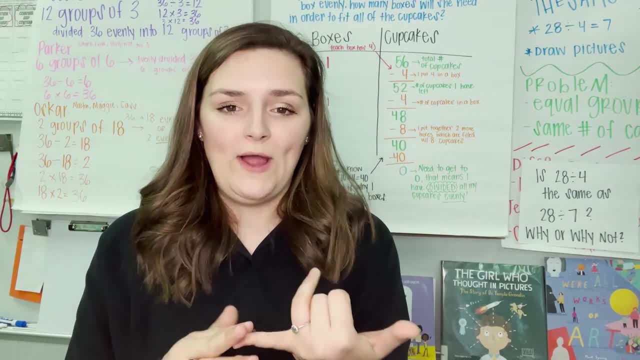 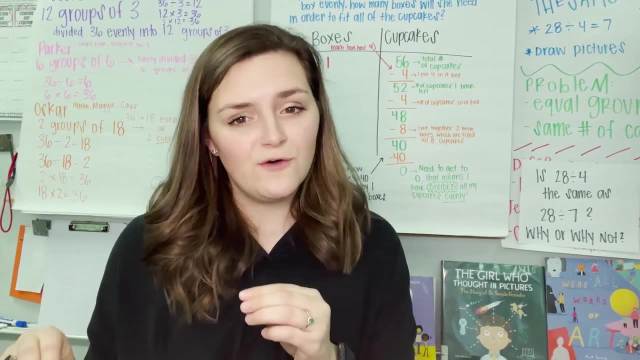 several matches, And so we were back to that whole practice test lecture, practice test lecture, practice test lecture and nothing was new And I really felt like a shell of myself And I thought: how can I teach math? 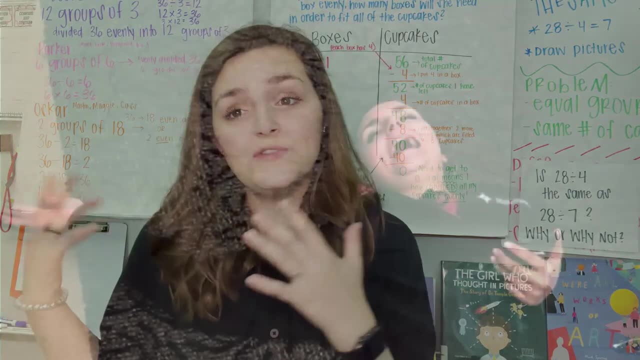 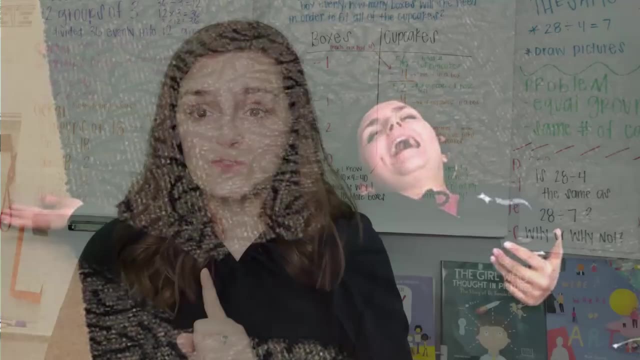 to others when I can't even do this myself. So that was really life-changing. and then I was like, wow, that dropped from scratch. And then I put all my math on hold and I think I was like, wow, that is so cool. And I was like, okay, this was. 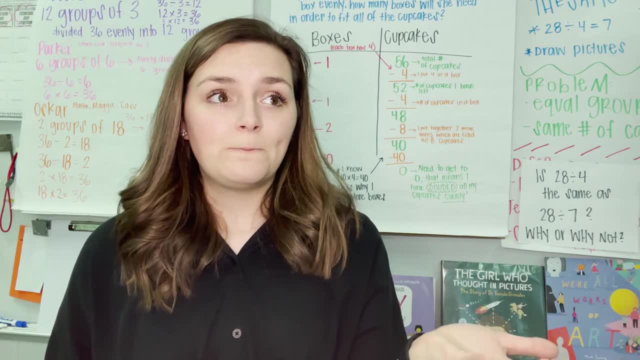 just my first time teaching math and I'm going to try my best. So that's some fast math Like that. doesn't sound like the best math that I could ever do, But I faced a lot of steps and I definitely had to learn math And I think it's really important to learn math because it doesn't 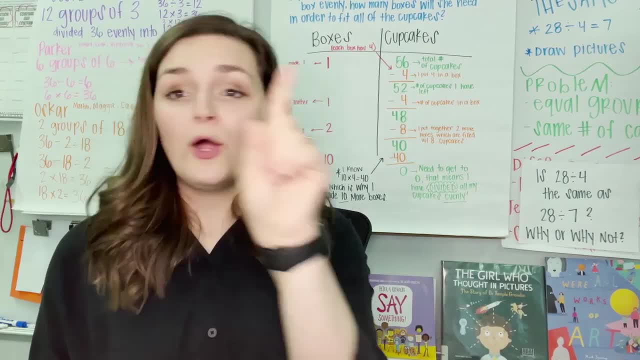 matter how good you are at math and how much you don't know how to do it, And I've always found that it is important to learn math because it's something you must have at school, And I've learned to learn math in college because I learned to know math and how to do math at school. 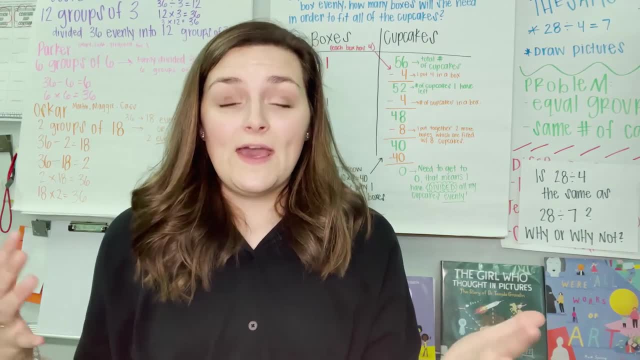 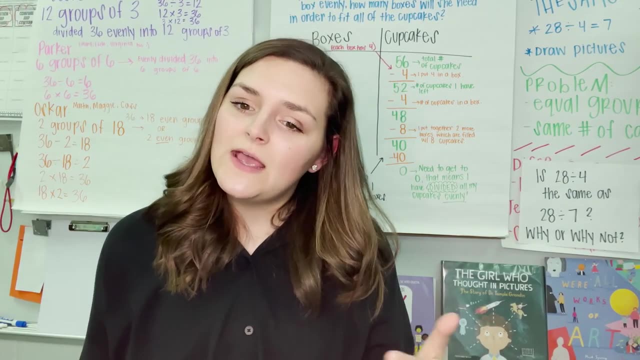 to you and mine just happened to be photographed and then put out there for everyone to see. I felt really inadequate and even considered dropping the ed major for a while because of this, because I felt that I could not teach math. I couldn't do it. We had two semesters of our math. 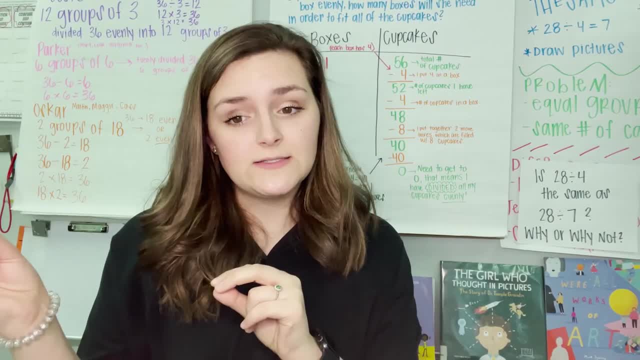 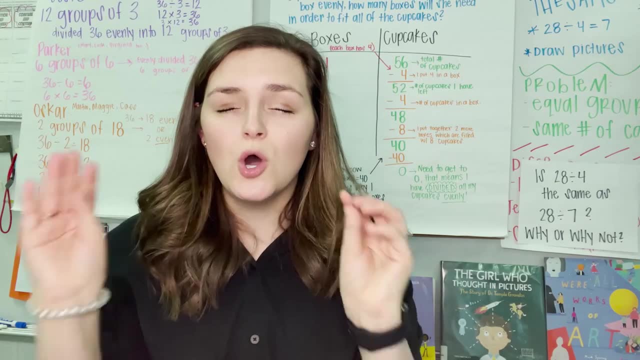 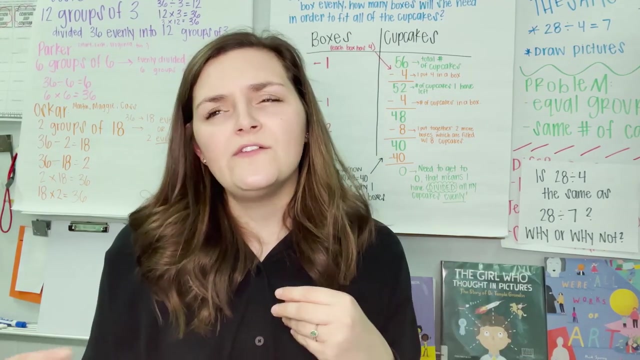 methods, class or, in layman's terms, how to teach math to kids, and I want to make this abundantly clear. Teaching math to kids is so different from learning math. The mental process behind it is absolutely different, and it's kind of like being told you can only use your non-dominant hand. 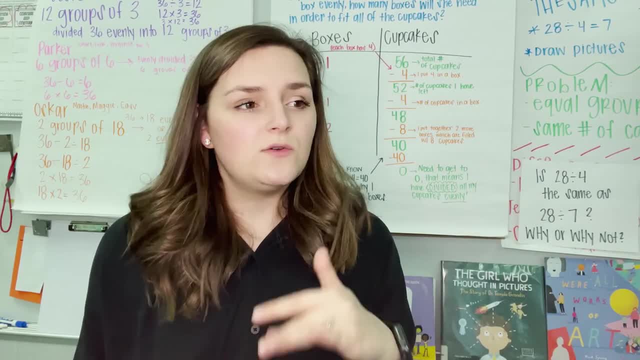 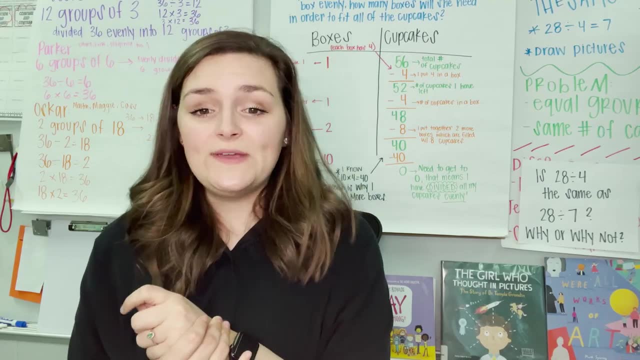 for the rest of your life. and these two classes here at Furman are taught by Dr Casey Hawthorne, who is a professor of mathematics, and one of the first activities we ever did was looking at this traditional algorithm of subtraction and addition, and I will never forget it. 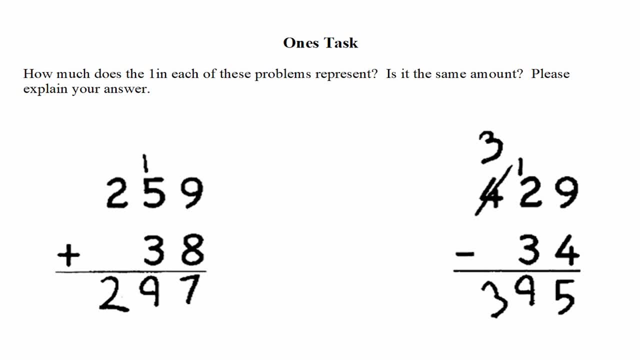 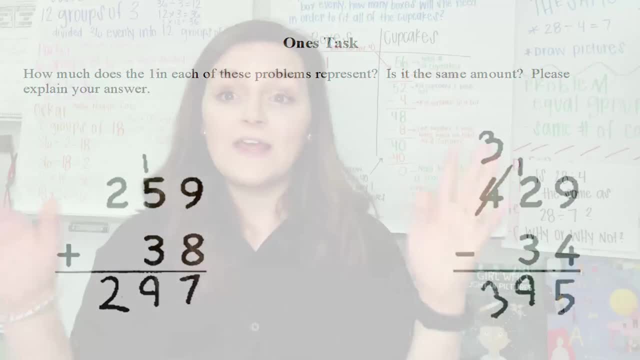 So we were asked to explain if the one and the addition and subtraction problem were the same. they represented the same process and did they serve the same purpose? Spoiler alert: they are different. So throughout this class we started to participate in these activities and they really 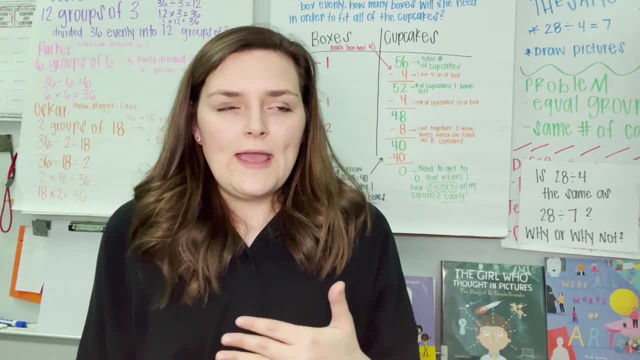 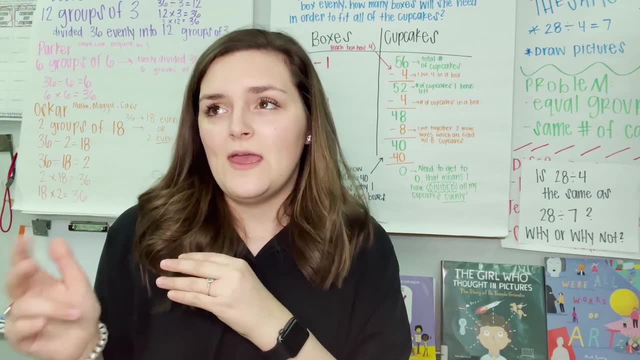 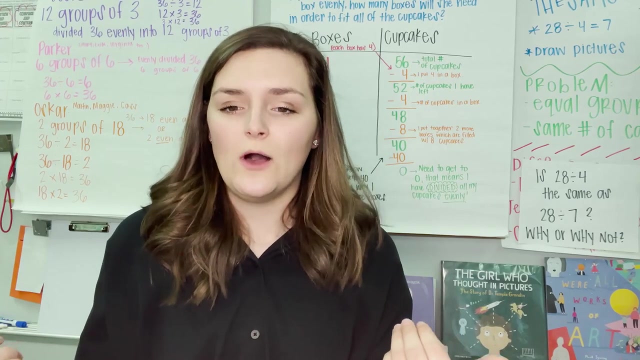 helped us to form our own number sense and fluency, and just like doing this one's task every single day, I started to feel a little bit better about my ability to teach math, and Dr Hawthorne encouraged us to really reframe our thoughts about who we are as mathematicians and who we are as teachers as well. and so we were told. 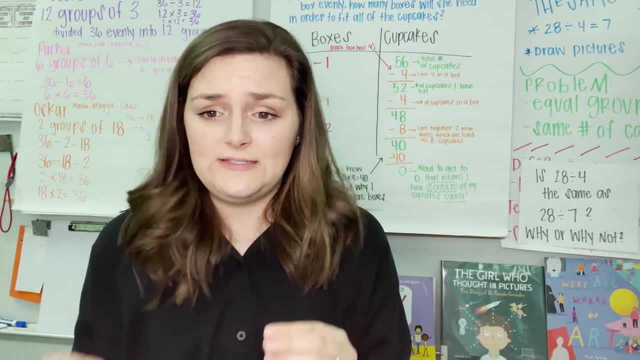 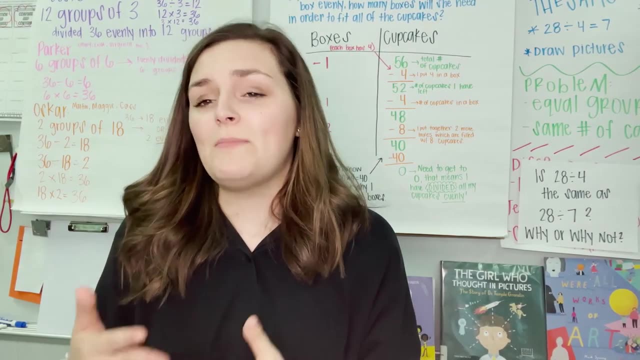 to tell ourselves that we are mathematicians and we can do these things. and as we worked on learning and participating in these activities and doing them as a group, I started to develop a better number sense and I really started to develop a soft spot. so with each activity we did, I gained. 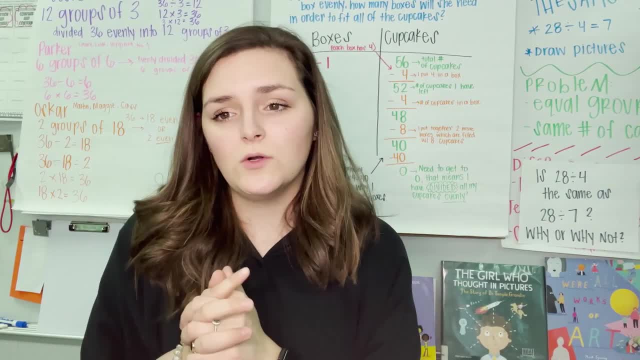 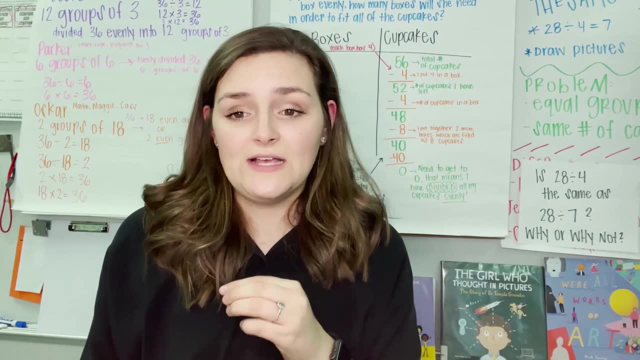 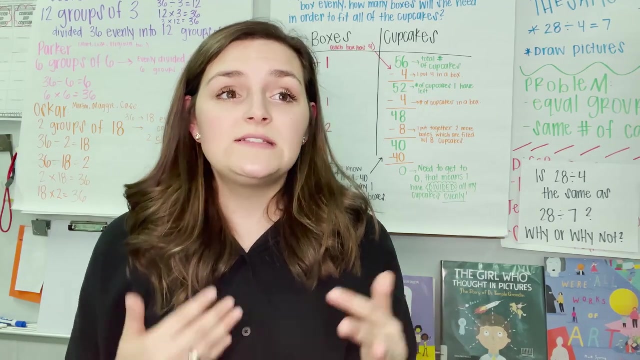 confidence, and some of these activities include number talks, choral counting and quick images which helped us to build our own fluency and number sense. So these activities are designed for students to participate in mental math strategies and then, while also encouraging whole group conversations, Seeing the positive reaction that my students have, 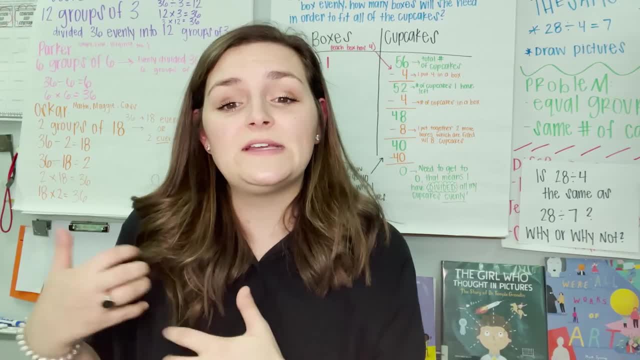 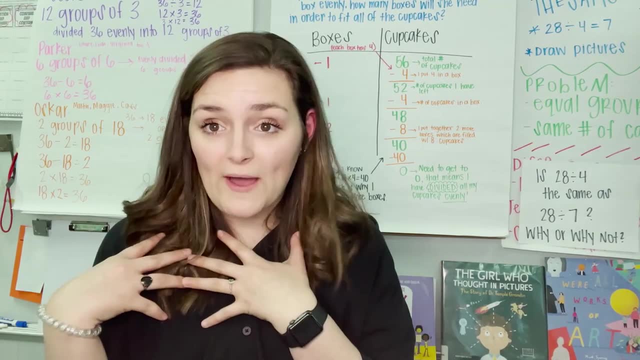 had to these activities has really made me crave the excitement to continue doing them and to really think of myself as a math person and my identity and that has changed as a whole and I am a math person and so are my students and that's important. Throughout my college career I have had the 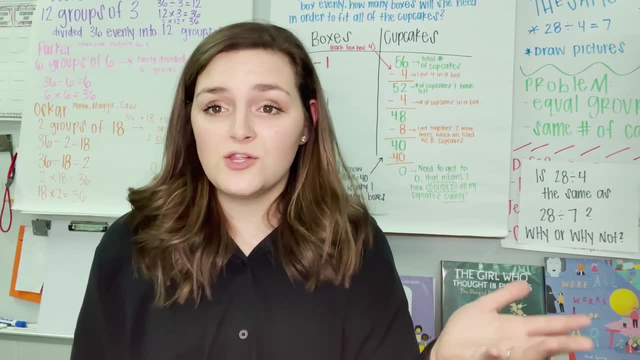 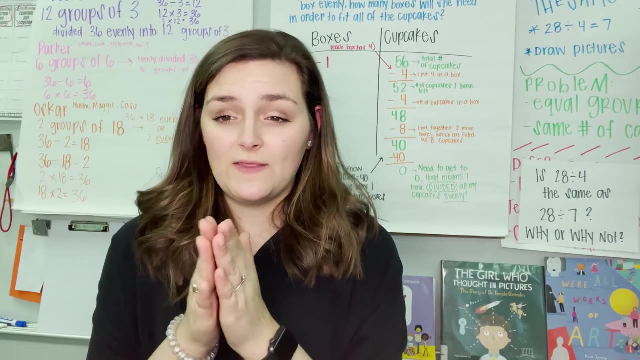 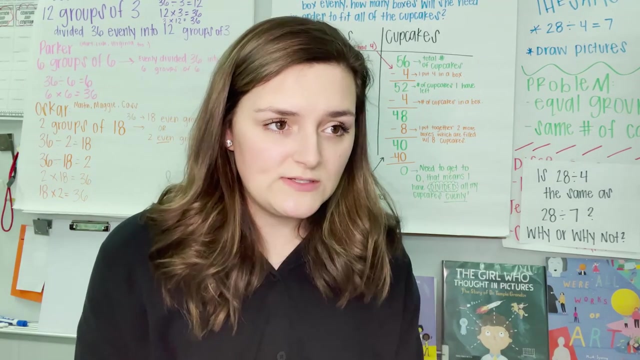 pleasure of working at an after-school program and done some private tutoring in addition to my field placements. One of my placements was strictly for us to work with a small group of students and implementing these new strategies that we have been learning. So the goal was for us to strengthen mathematical fluency, boost student self-confidence while 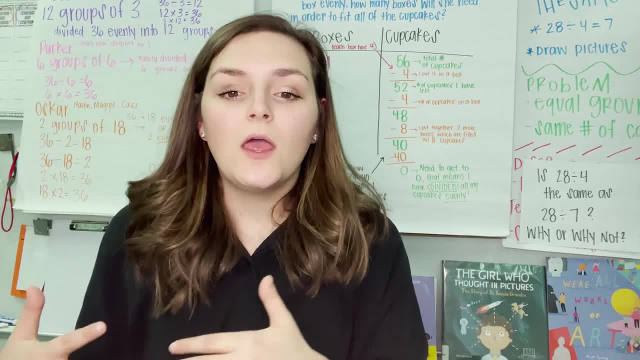 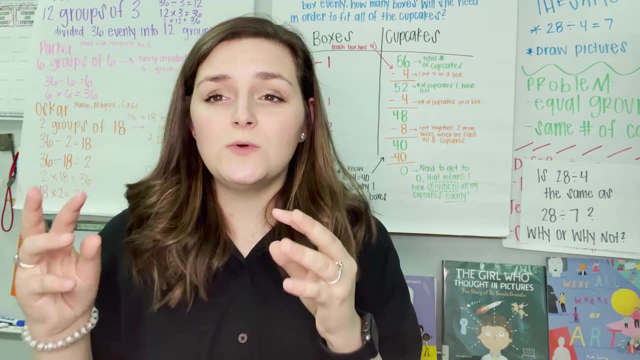 also giving them a positive self-identity when it came to math. Before we interviewed them, we started to role play and do these different things to help us prepare and to just do a little bit of background on these students and see how they're feeling. 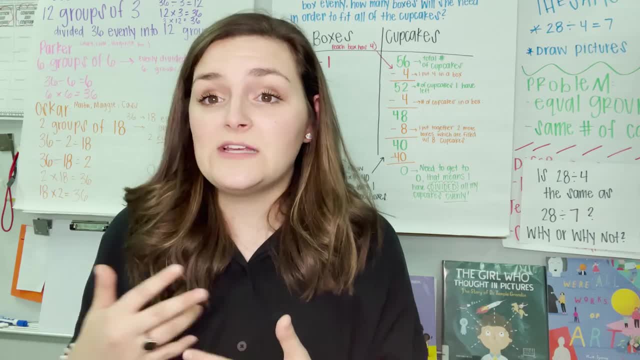 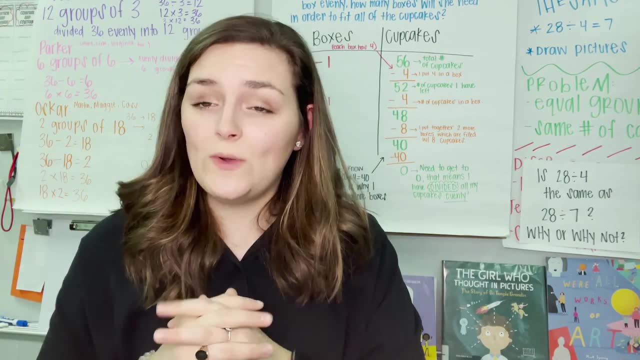 So before this, we did some role play to help us understand what it would be like to interview these students, and nothing could have ever prepared me for what came out of the student's mouth. We'll call him Carter. So we asked: Carter, how do you feel about doing math? What do you think about? 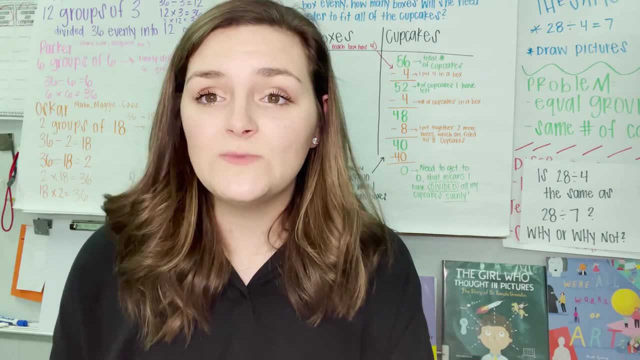 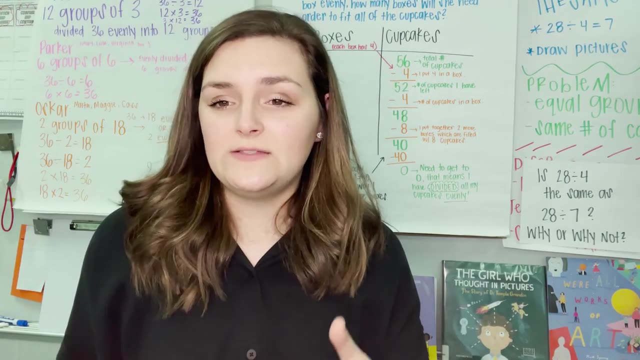 that Carter said, I feel like a demonic spirit is inside of me screaming: Wow, what, what do you do? What do you? how do you respond to that? My partner and I, we just kind of looked at each other in utter and complete disbelief. 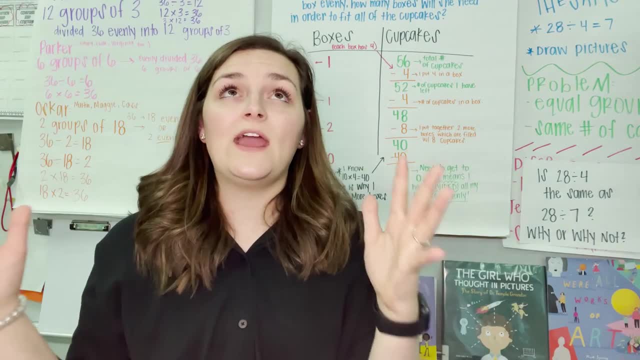 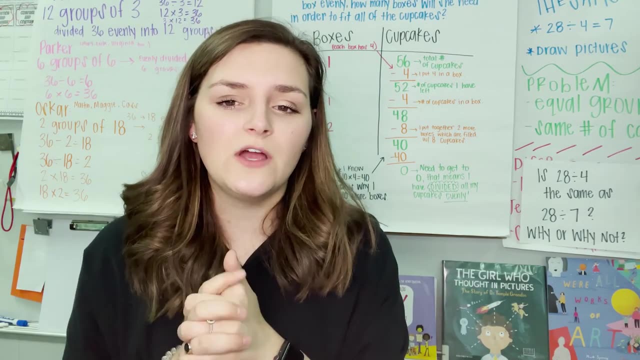 This kid hated math more than I ever had in my entire life and he had an extremely negative view of himself, and an extremely negative view of himself when it came to math especially. Another example is from when I was working with one of my favorite kiddos, and we'll call her Jade. 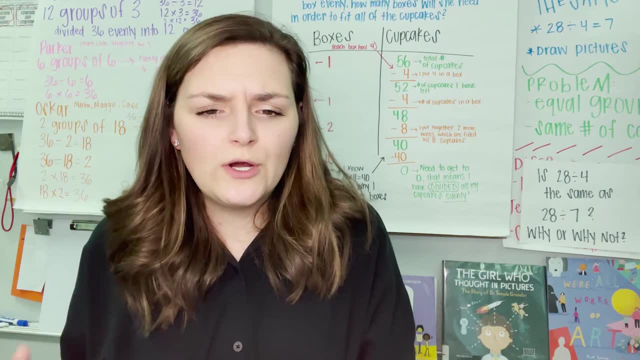 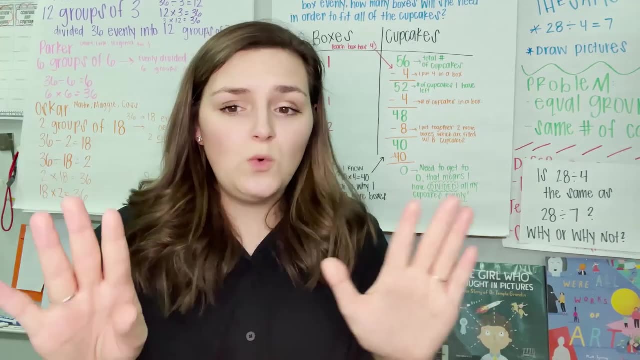 So Jade and I have been working together for a while. you know, every time we start to work on math, she immediately would start to cry, and she would just shut down and say: I can't do this. math is too hard and she doesn't know how to do it, and so her actions reminded me a lot of 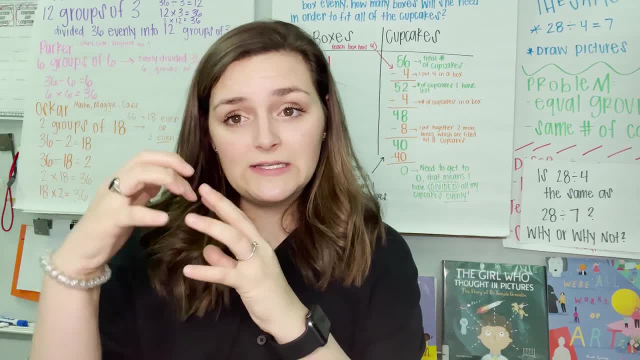 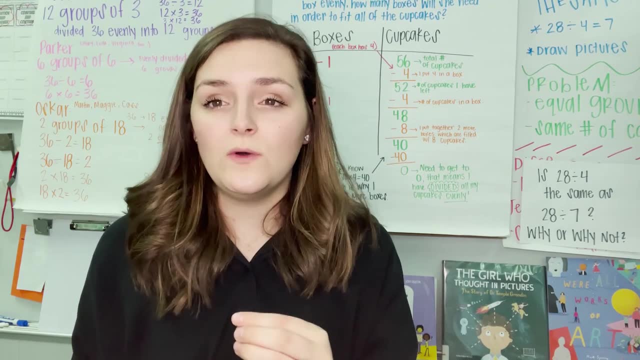 sadness from inside out when she would just melt into a complete and inconsolable puddle. Jade said our teachers moved too quickly, they always marked her answer wrong and again she had a very negative self-view of what it was like to be a mathematician and have herself connected to. 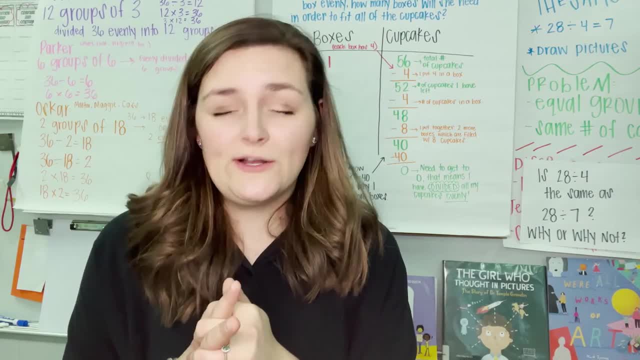 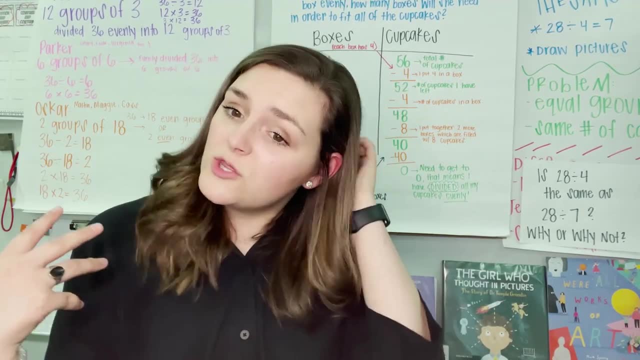 math. Another student I worked with was having very little understanding of what it was like to do a division strategy. her teacher taught her earlier. so she came to me in the afternoon and we just were working on this and I took it upon myself to teach her a new method that I thought. 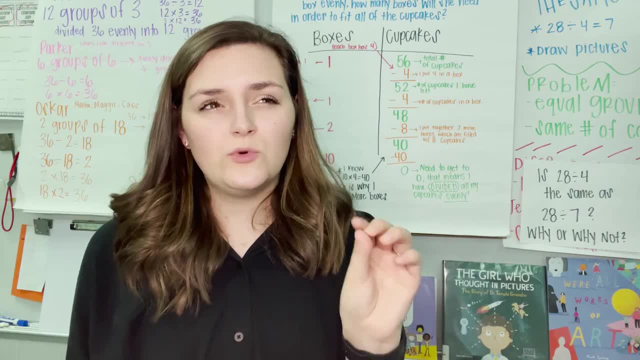 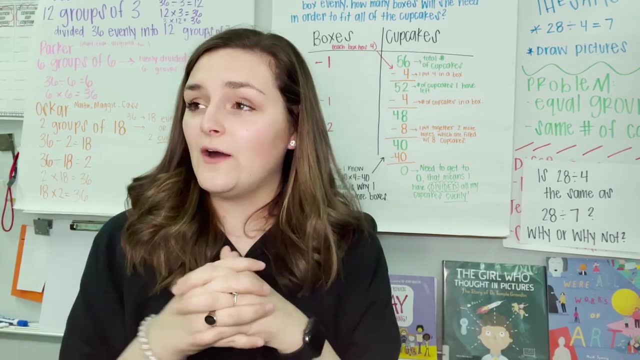 would be helpful and she really got the hang of this method and was really excited to go the next day back to school. but instead of this, her teacher emailed her mom and asked her mom to ask the tutor to stop teaching her different methods what were being what was being taught in school. 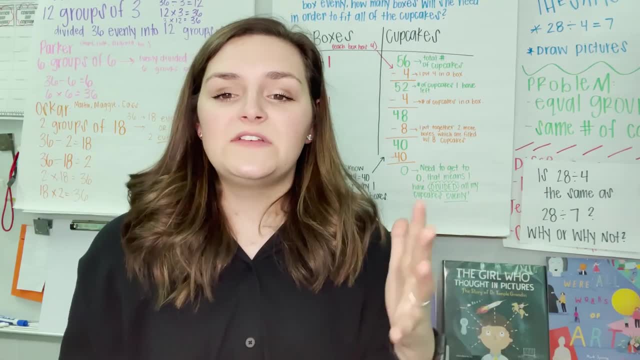 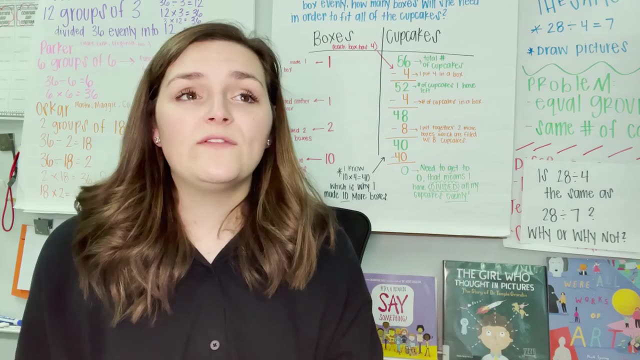 and so I was completely shocked, completely. this teacher shut down her ideas and this child's confidence in a simple one-handed swing. so her mother said that she was crying all afternoon. at least, that's to completely redo the homework that they had done the day before, and she was. 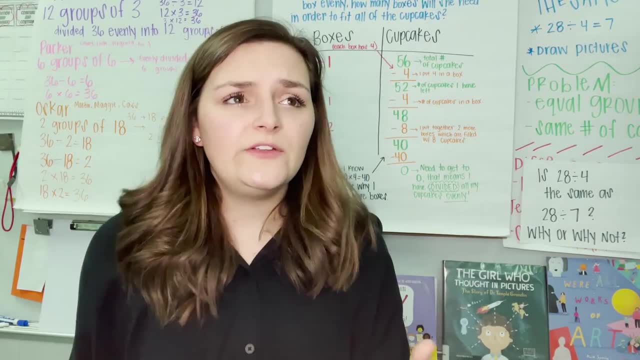 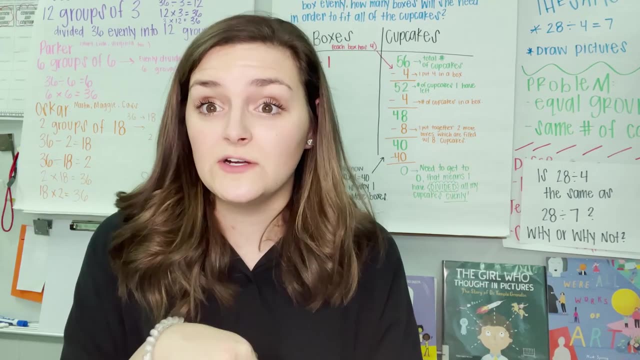 absolutely devastated and so telling you all of these horror stories. I tell you this because I want to tell you about some of the amazing work I've been able to do with my students thus far this year. so I'm currently placed in a local elementary school here in Greenville and I work. 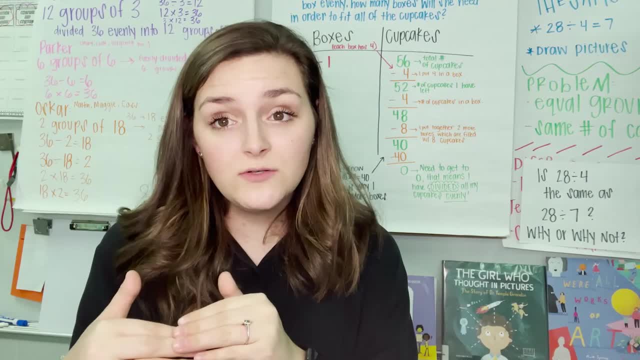 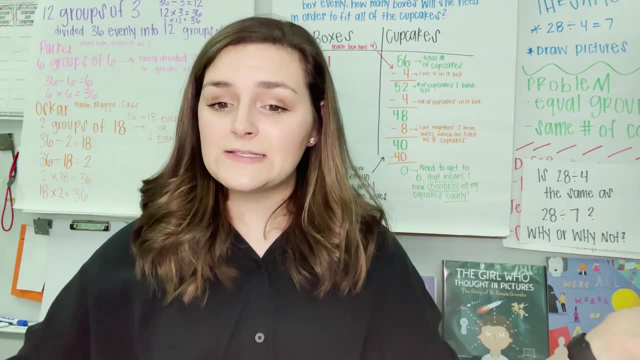 with multiple grades, but I specifically work with fourth graders the most, and so those are my kiddos I want to highlight. if I had to sum up the basic things I see from my students, this would be it. so i've got different types of students, as most people do, and i have some who 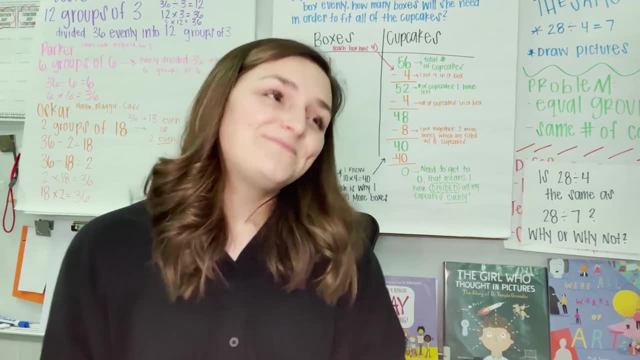 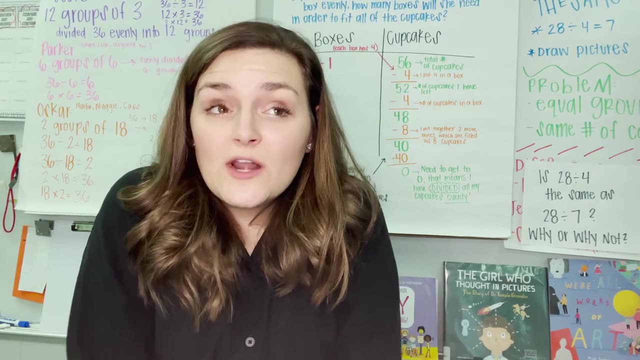 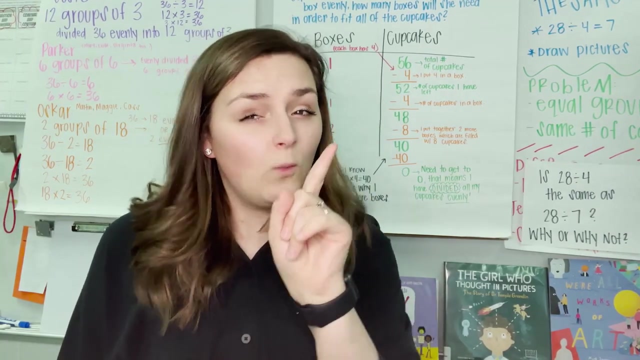 wait for someone else to say the answer so they can just nod along in agreement. i have others who look at you with a completely blank stare. and then i have those students who shout out the answer every single time, even though you've asked them not to 500 million times. and then there's that one student who's aggressively. 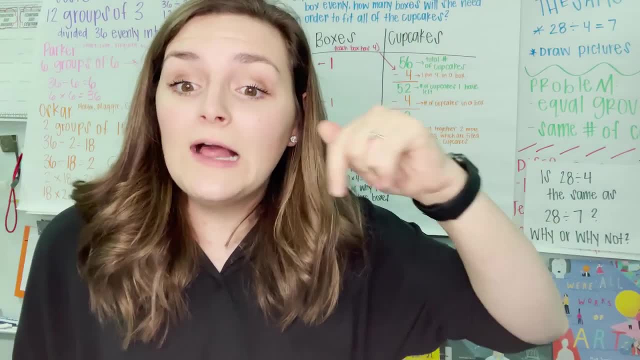 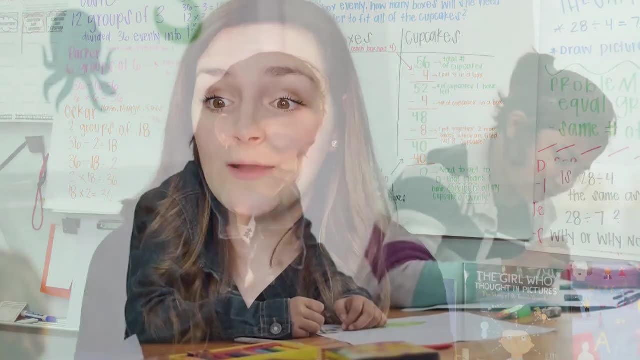 making eye contact with you and raising their hand aggressively, aggressively, like the world is depending on it. and when you walk by their desk, they're talking just a little bit louder just to be sure that you can hear them, and i know you're all extremely surprised to hear. 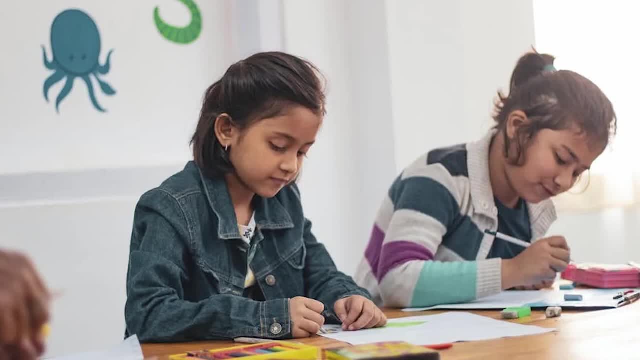 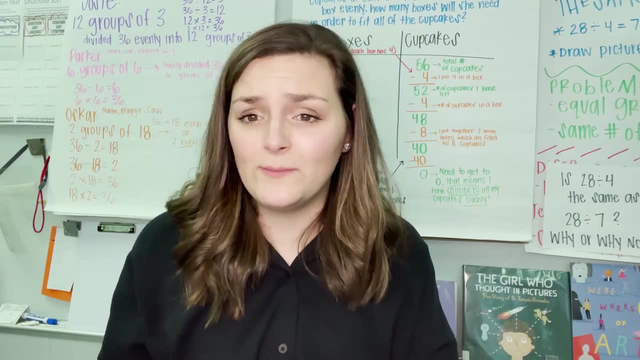 this, but that was me as a student. that's who i was as a student, so i'm sure that all of you have fallen under one of these categories at another point in time. so my question to all of you now is: what do we do with all this information? how do you teach kids when every kid is so different? 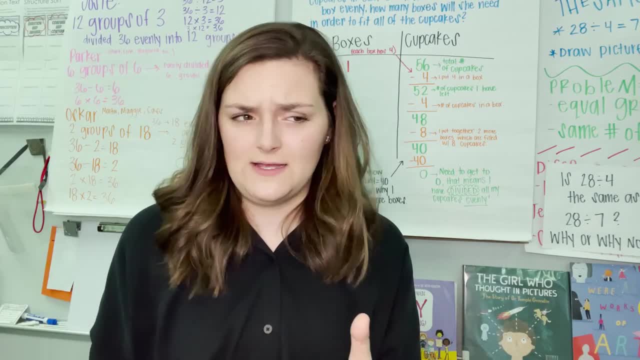 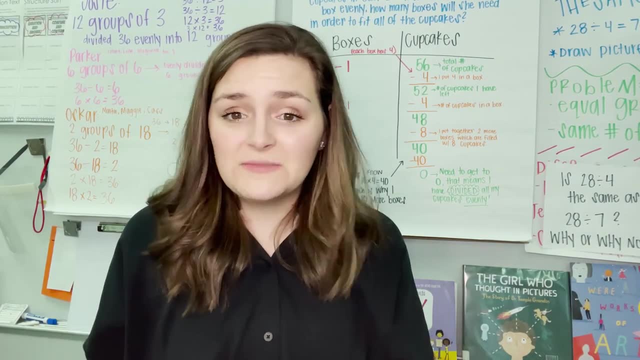 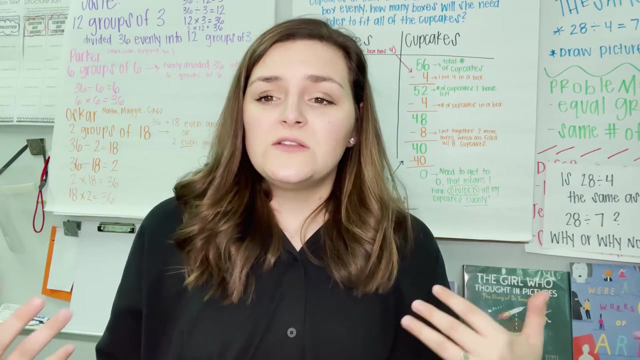 grown-ups and their kids are constantly having battles over math. how do we fix this? how do you teach students to be confident and create deeper meaning with math, all at the same time? and, of course, i don't have all of the answers, but i do have a proposed solution, and so i believe that, if we are 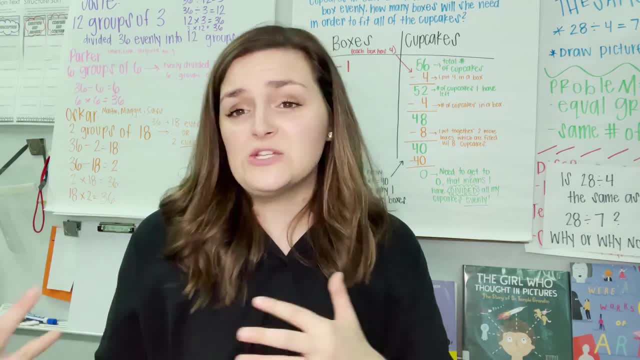 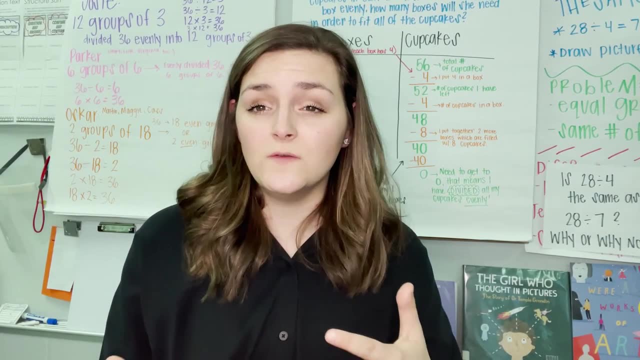 to integrate these different methods into teaching into our classrooms, that we're going to start to create a deeper meaning and understanding and create a positive view of have students create a positive view of themselves as mathematicians. i know this works because i've seen it in my class. 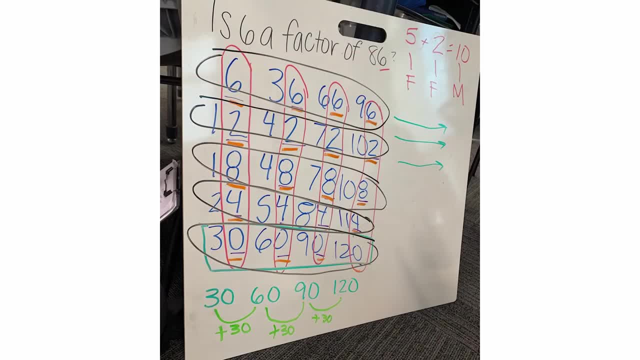 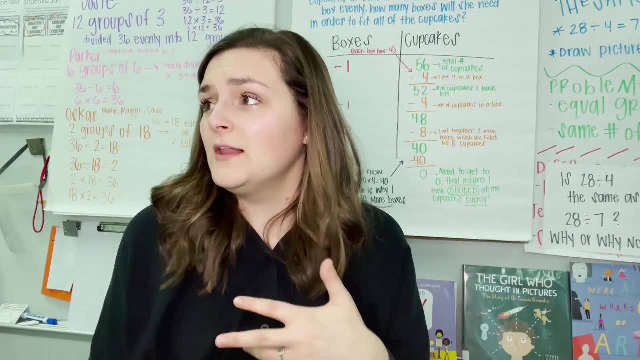 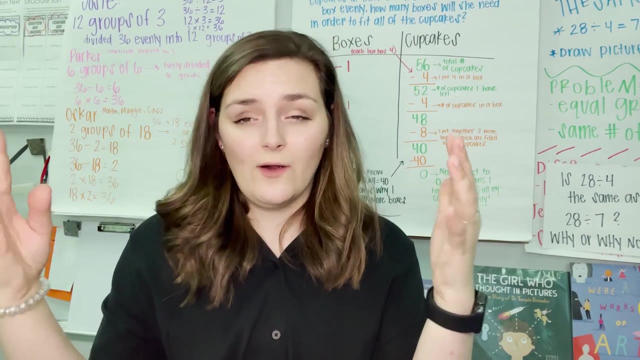 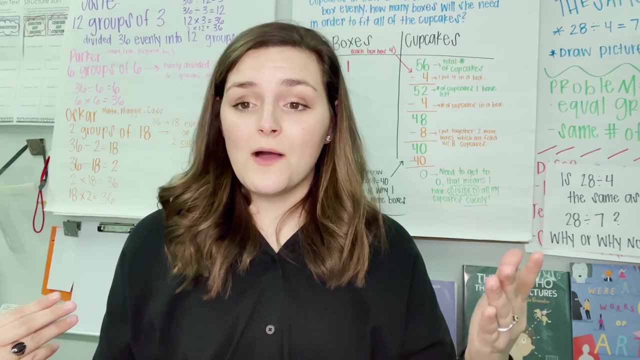 firsthand my fourth graders clear their desk and frame their subjects in their classrooms. you know, i just like your guide and kind of have this interactive spirit that you can connect with them and make them feel better. um, and then everything started with a little more than just one same person. 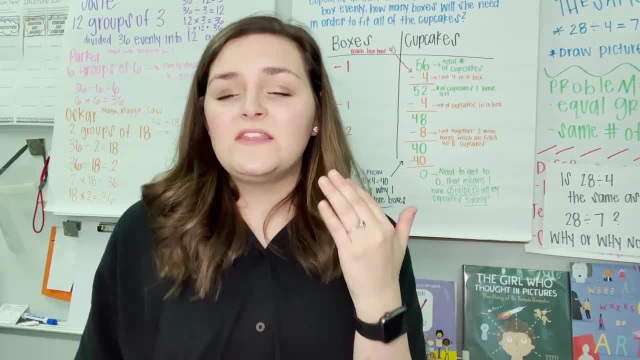 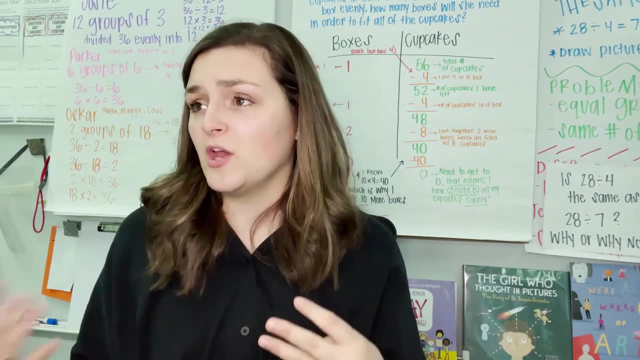 Overwhelmingly. all of them said that doing math with me made them more confident and they no longer felt pressure to get the answers right And more they focused on being able to speak up and share with their friends and have a conversation as a class. 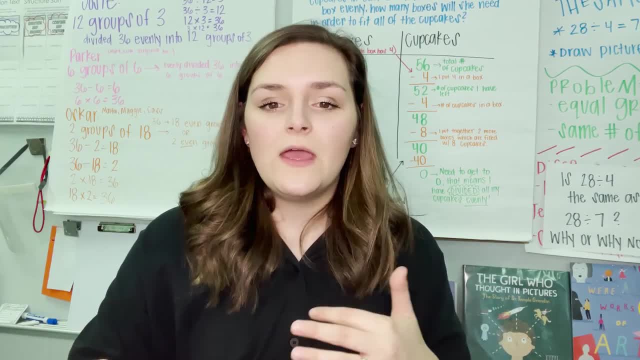 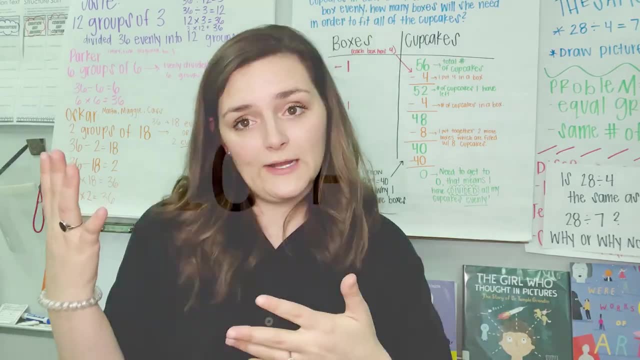 And they felt that they had created deeper meaning within these activities that we were doing. So some of these activities I wanted to share with you today. The first one is a number talk. So if you look at this problem right here, it's going to flash up on your screen. 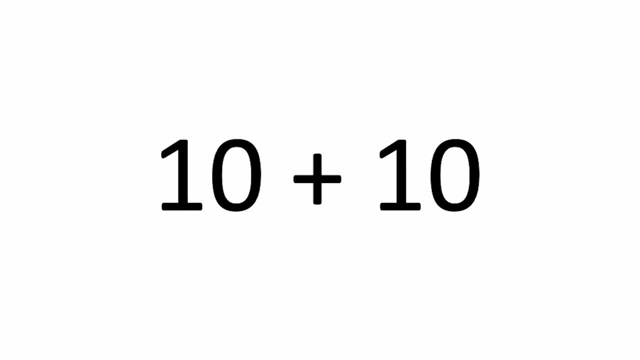 It's 10 plus 10.. So I start by putting this on the board and I would give you a few minutes to solve this problem, And so, once you've solved it, I invite my students to try and think of another way to solve it. 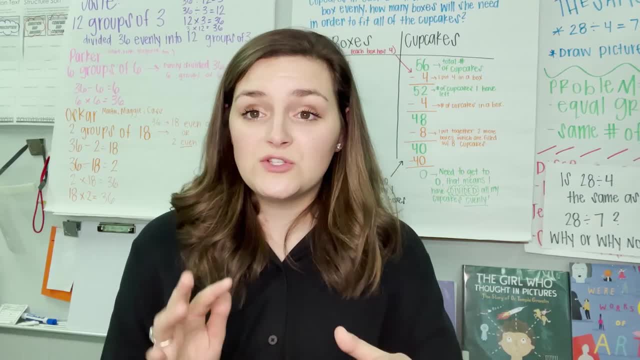 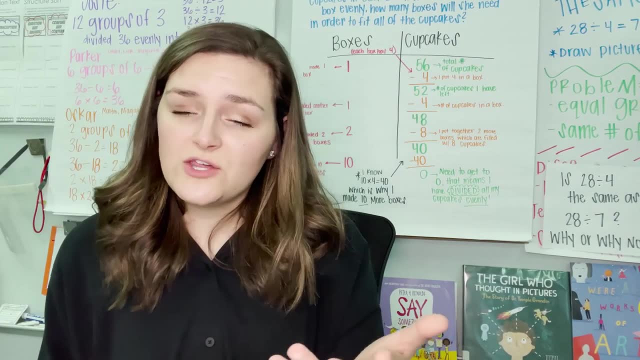 Following. we're going to have a few students share out and my students are going to turn and talk with each other and with a partner to discuss ways they have solved this problem. So we're encouraging those conversations while also honoring student thinking at the same time. 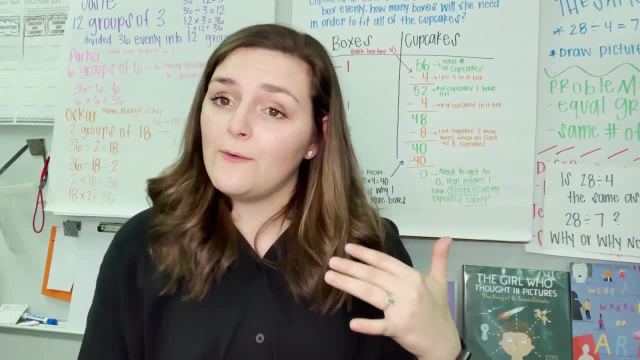 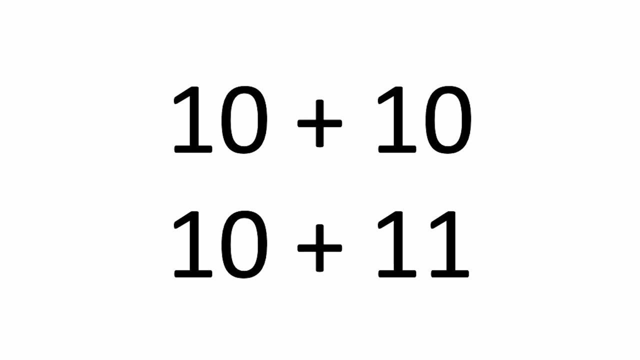 Following this, I would write another problem on the board directly below that one. So this one is going to flash up on the screen. It's 10 plus 11. And so I encourage students to use what we did in the first problem to help us with this next problem. 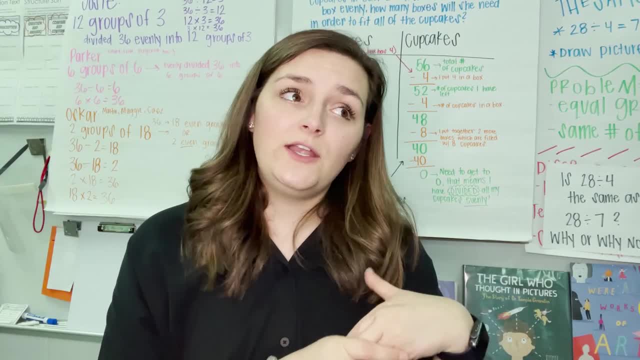 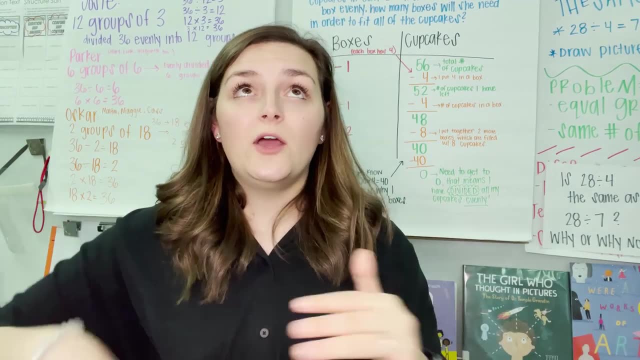 So if you solve this one using I know, if I break up 10 into two parts, it's five plus five and I have two tens of five plus five plus five plus five is 20.. And then I know I have 11 in this next problem. 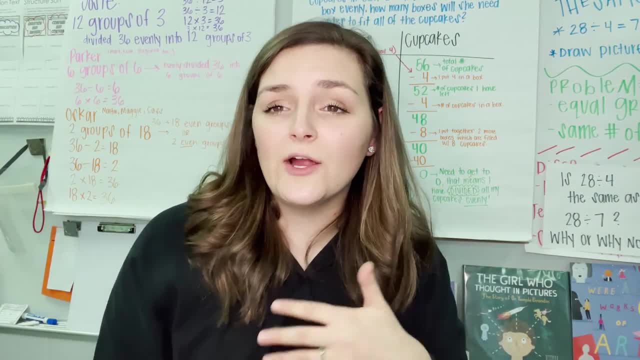 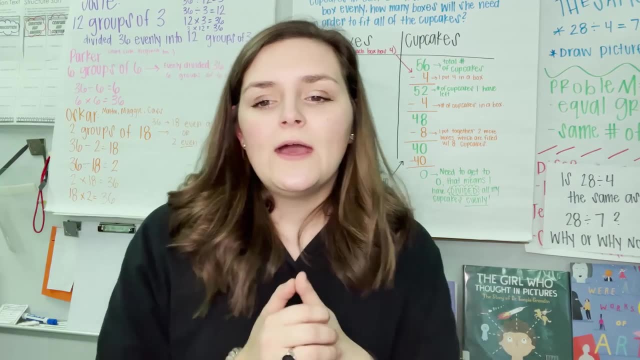 I can add one more to make 21.. So each time we are going to add a new equation to this and I would give them time to solve it independently, try to talk to a partner and then have a whole group conversation together, And this is allowing our students to learn from each other in the process. 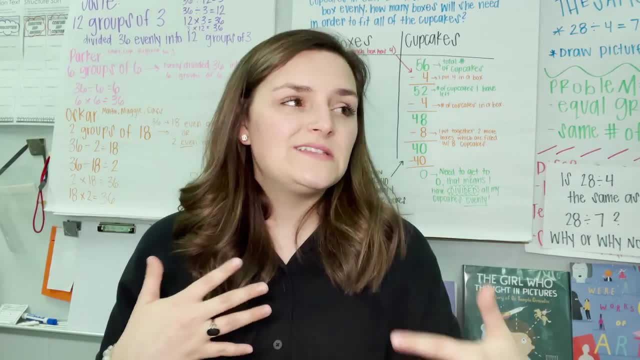 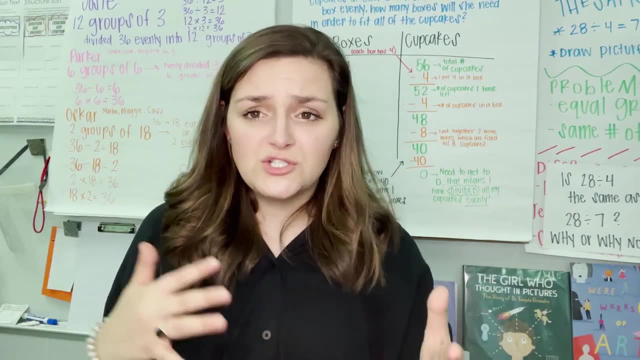 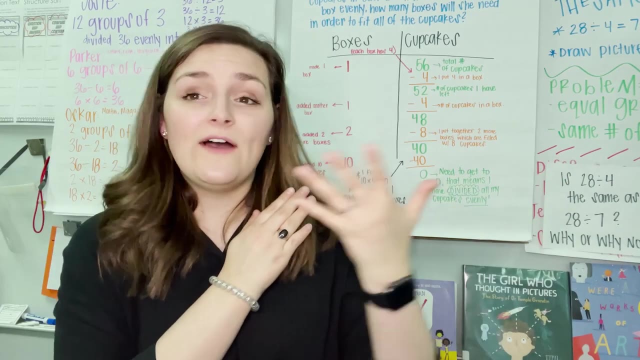 Another component is re-representing student thinking. So, for example, some of you may have said five plus five is 10.. I would write that on the board in a different color for students to be able to see that represented. It's a very key strategy for students to be able to see their thoughts put into a visual and have it actually represented on the board. 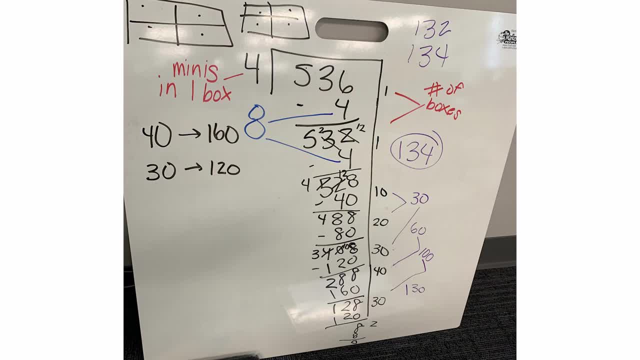 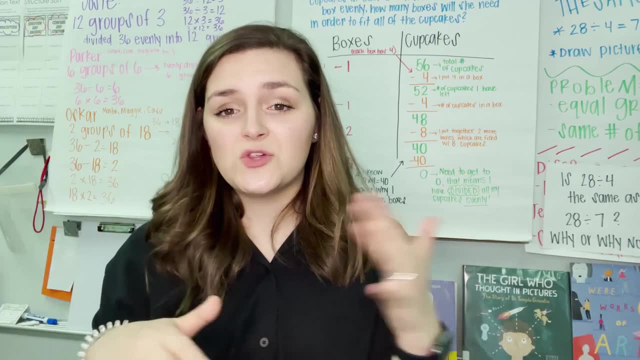 Representing student thinking is a key strategy because it's allowing students to see their thinking visually and to actually see it up on the board. And so we could continue to add equations, going on And on and on, to see connections between the numbers. But I'd rather show you a different strategy. 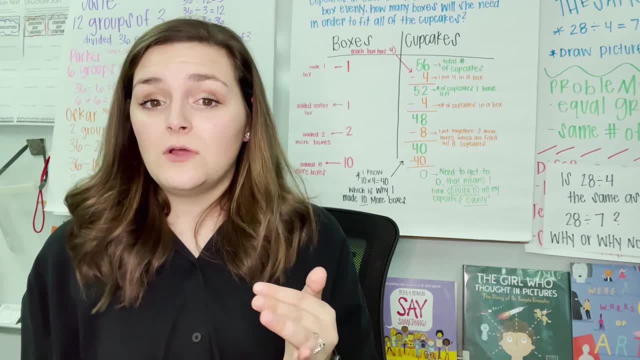 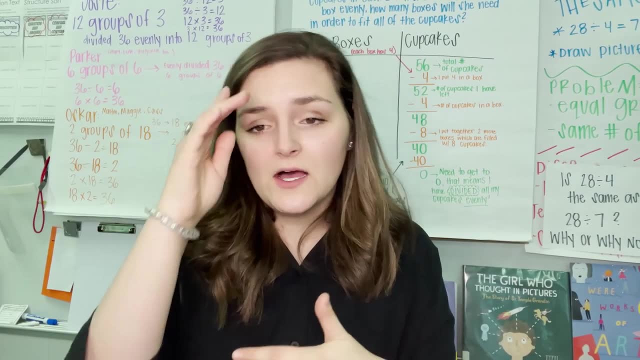 So this one here is called choral counting And basically we're just going to skip count by a number and keep going, And we're going to have the whole class do it in harmony. So it takes a few tries for everyone to get it as a whole group. 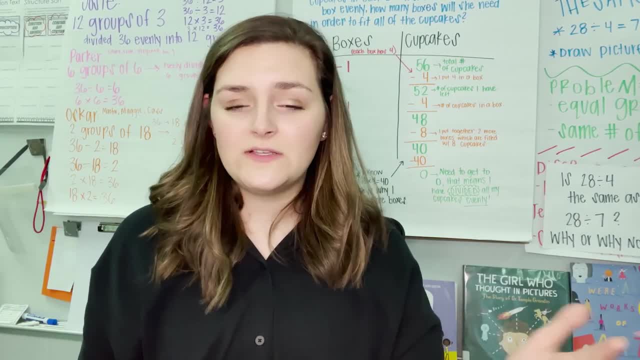 But we would start like this: If I would say we're going to choral count by fives, we would go five, 10, 15,, 20,, 25, 30. And then we would stop and look for patterns in this. 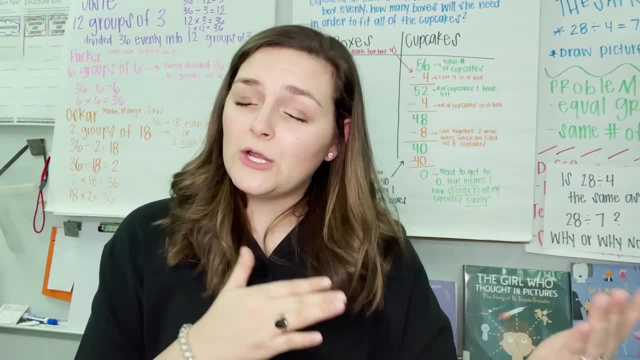 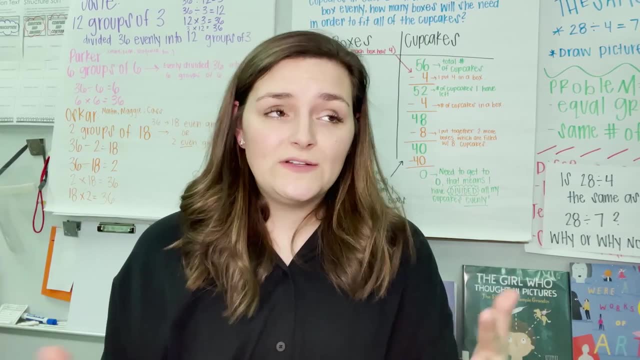 And again, students would first think to themselves And then we would encourage, turn and talk And have a whole group conversation. So seeing these patterns helps students to make connections between numbers. In addition, it helps students with multiplication and creating factors and all those different types of things within these numbers. 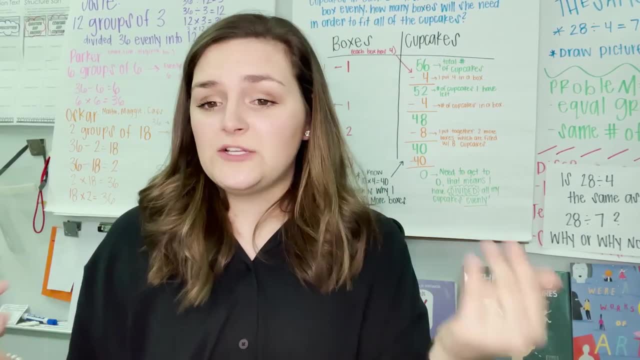 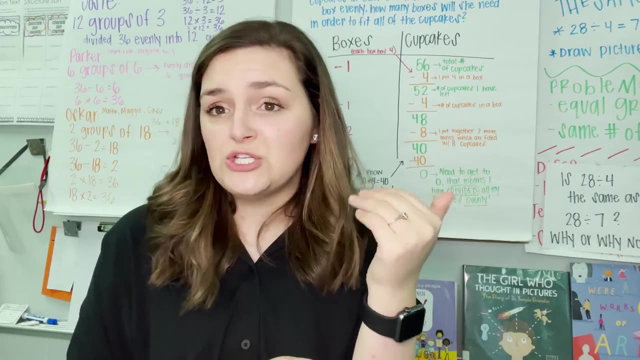 And the best part is, you can literally skip count by anything. I can skip count by twos, by fours, I can even skip count again by fives, But starting at five and going 12,, 17,, 22,, 27 and going from there. 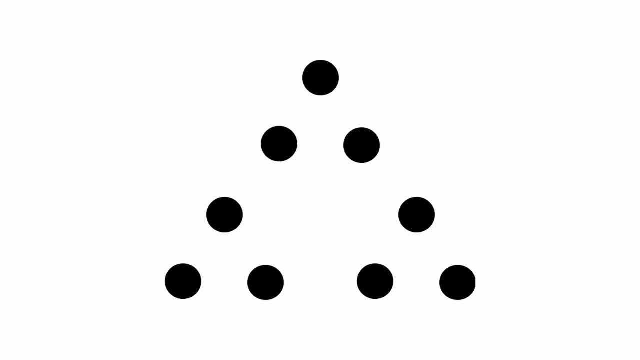 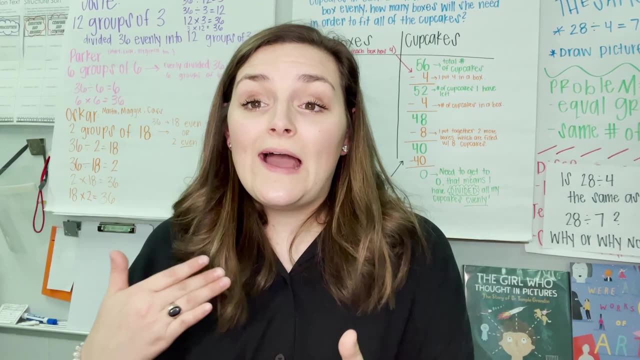 So another strategy we use is a quick image, And here is an image of a quick image, And again, I would ask my students to tell me something about this, And then I would ask my students to tell me something about the image that you just saw flash up on the screen for a second. 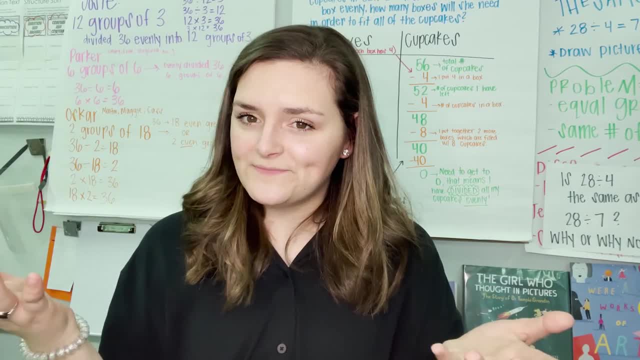 So this one is: how many black dots did you see? And then I would show the picture again here, And then I would ask students to see if they begin to see a pattern. And so, of course, you guys are probably beginning to see a pattern here. 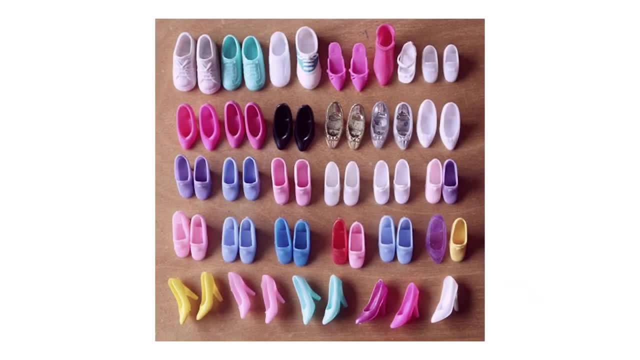 But it doesn't just have to be done with dots. It can also be done with real world things, like these Barbie shoes. We can look at a fraction that is pink or how many pairs there are, And this image could use several different factors. 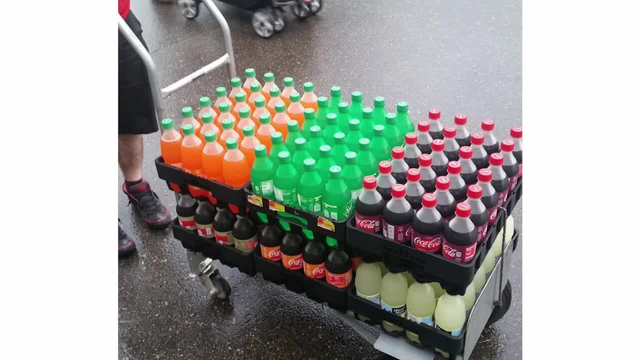 So this is another example right here that I've used with my class, And it's about soda bottles, And we wanted to see how many pairs there are, And we wanted to see how many pairs there are And we wanted to know how many total soda bottles there were in total on this cart. 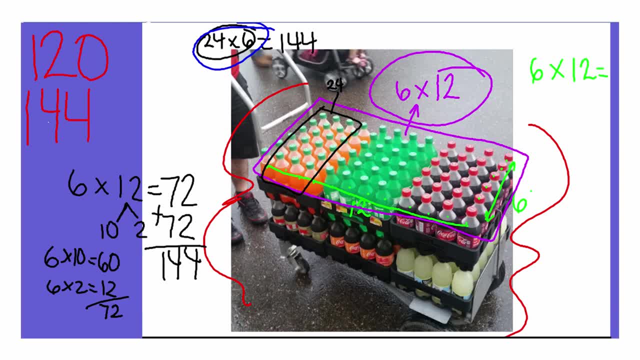 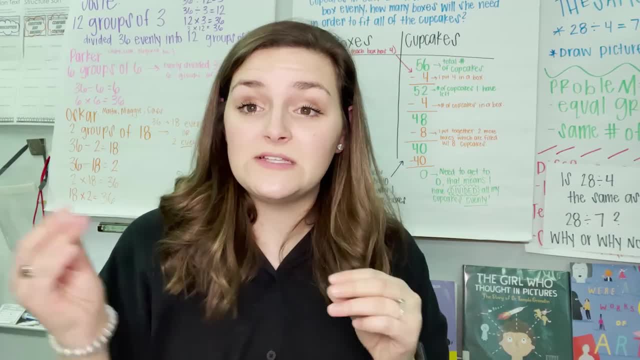 So we started with this image and we ended up with this. So all these different colors in this image are different ways my students had thought about these different strategies or what they had used, And so that was a powerful thing for them to see their thinking represented within these.